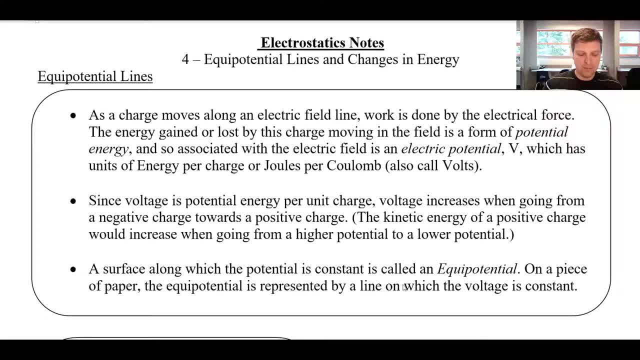 and it's a little bit strange. So a couple things to keep in mind here, just a few bullet points to think about. If you have a charge that's moving in an electric field, we said that, for example, the direction of an electric field line would be the direction that a proton would want to move in that. 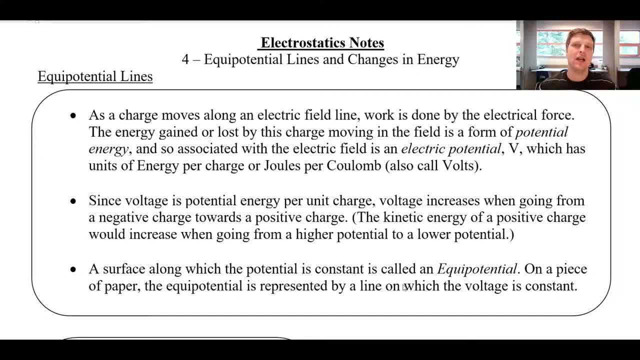 field. So if you have a proton following some electric field line through a field, then work is being done on that charge. So, as it follows the field line, we're doing work on the charge. and if we're doing work, then that means that the potential energy of that charge must be changing. And so, as 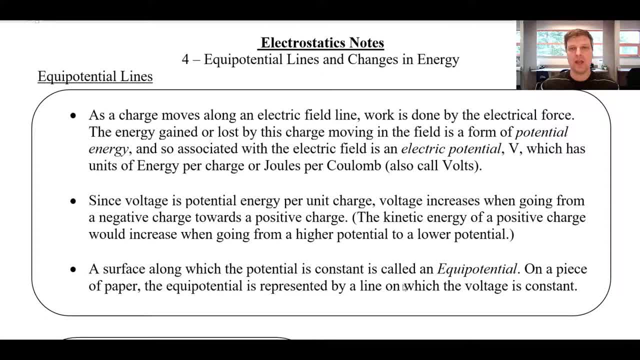 we move charges around, we're changing the potential, energy, and this relates back to this idea of potential, because charges or fields have areas of high- if it's a positive charge- or low potential. And so if you move another charge around in that electric field then as you go from, for example, take a proton from low to high. 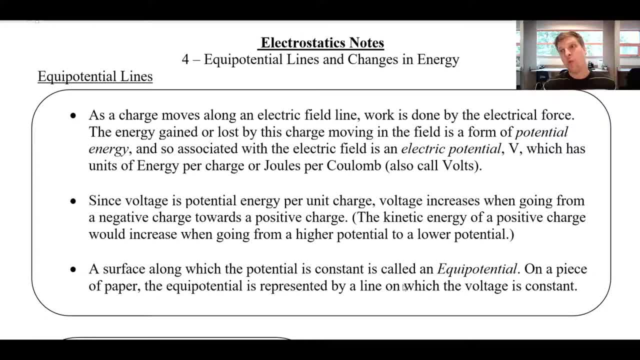 potential. you're going to be increasing its potential energy, You're doing work on it to move it up to an area of higher potential. And so a reminder: voltage is this: energy per unit charge. It tells us how much energy per unit charge we have. 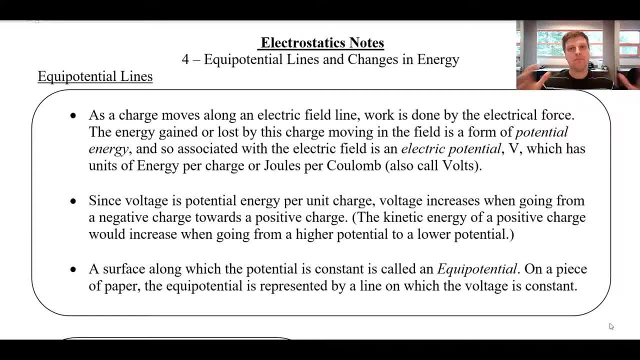 And so if we have a surface, if we have a space and we're trying to describe how the potential changes, we're going to use this idea of equipotential lines, And equipotential literally just means equal potentials or equal voltages. So when we draw, 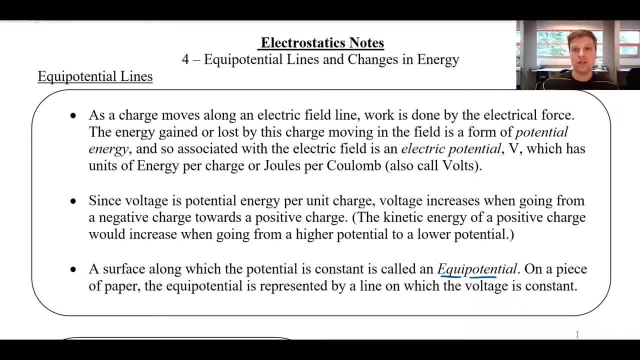 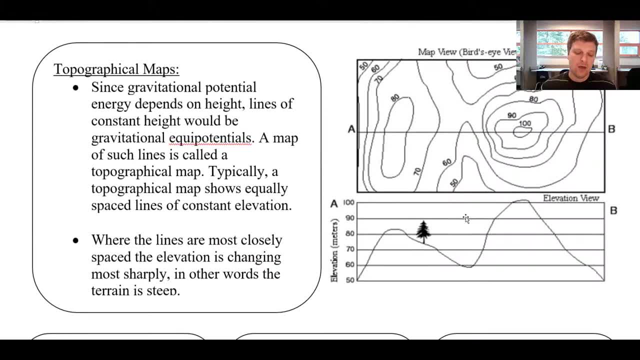 lines on a piece of paper and it's an equipotential line. it's showing a region of space that has the same potential. Now, an analogy that I think is going to be super useful when we think about potential as it relates to for. 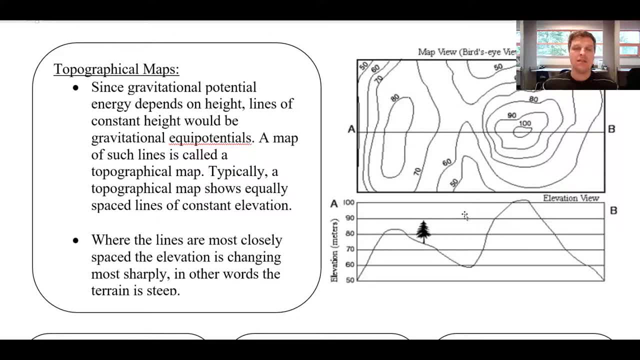 example, gravity, Like what's the going on? there is to think about these potential lines as kind of topographical lines, And our potential is going to give us an idea of height. So if you look at this map here, this is something called a topographical map, If you want to draw a bird's eye view of a space, and 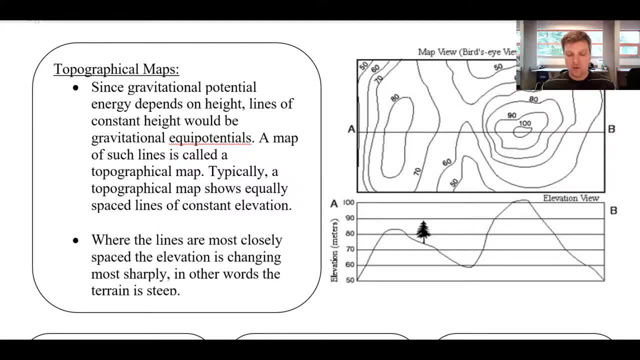 you've got mountains and valleys and things going up and down. if you want to represent those, you might draw these topographical lines, And what that means is you can see here from the side view. in this space I've got kind of a smaller mountain and then a. 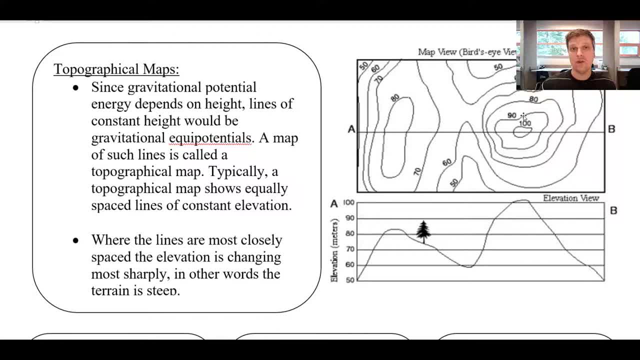 bigger mountain. But if I draw the vertical line here of the shape of mountain and then the vertical line over here, I can represent the height of that surface. So these equipotential lines. you can see this line here that says 90, you can imagine if I walked all the way around that line that'd be like I was walking around. 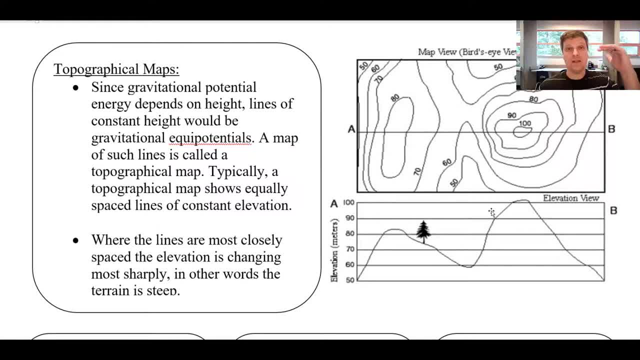 this mountain And it was staying at an elevation of 90 meters. So I'm staying the same height above zero. I'm staying at the same potential And, in actual fact, if I was to walk around in a circle, I wouldn't be doing work because I'm not changing my energy. If I compare the four elements, 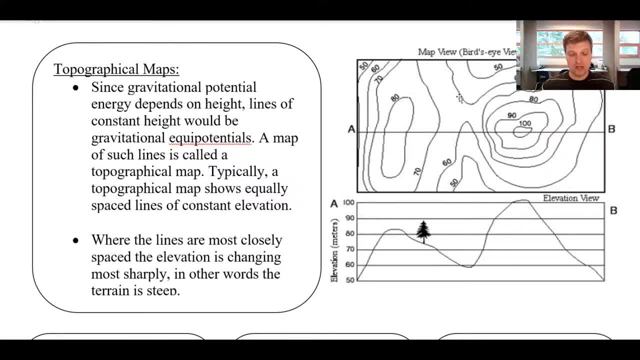 climb up to 100, well, in that case I have done work. or if I roll down the hill to 50, I've done work as well. So we can think of electric potential as kind of like being height, where positive charges kind of make mountains and they make really high areas of potential and negative charges kind of 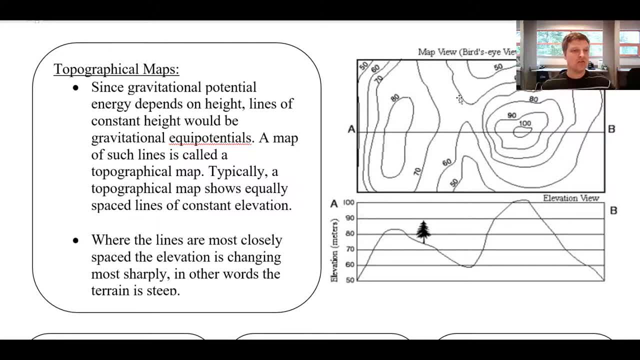 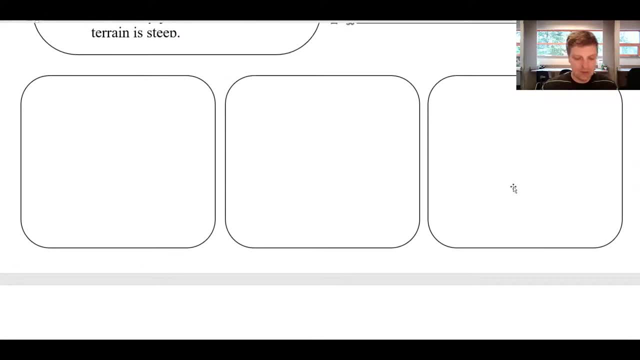 make valleys or areas of really low potential. and you can imagine if you have multiple mountains, well then they would just make multiple areas of high potential and so on. So we're going to try and visualize this here. we're going to do a little bit of like a visual experiment, where what would 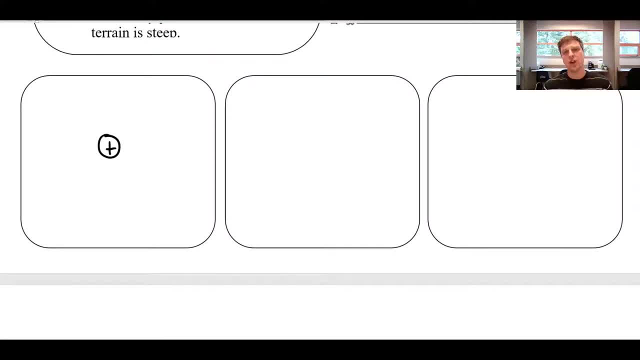 it look like if I have a a positive charge sitting in this space, just one single positive charge, and as a reminder, you could think of this if you like, I'm going to draw the side view first, whatever that means, a side view of our charge. but it's kind of like a region where we've got a really 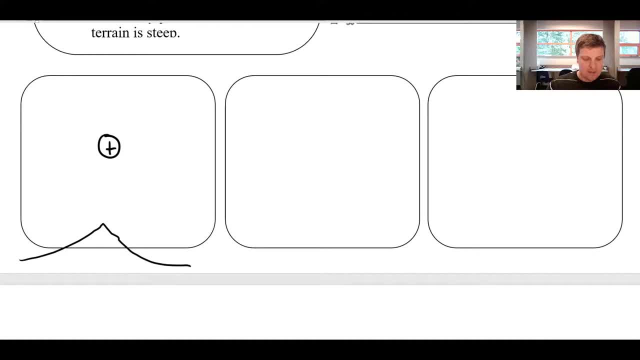 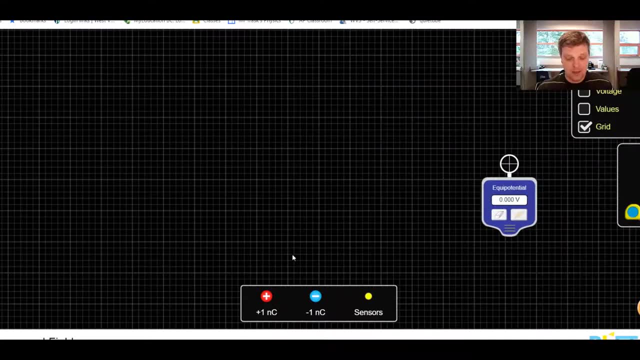 high mountain right. so it's like this high mountain peak in the center, and so what will the equipotential lines look like surrounding that? I'm just going to use this really handy, this FET simulation That kind of shows this. so if I have a single positive charge, we can see the electric field. 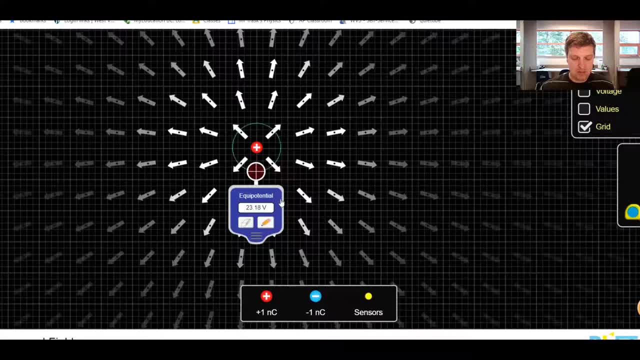 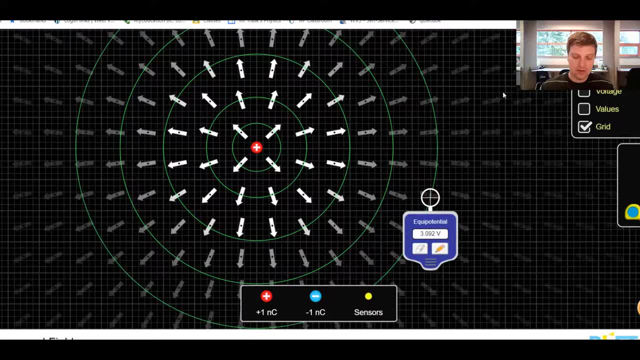 surrounding it. if I go close to the top of this mountain and draw an equipotential line, you can see that it would be a perfect circle. and as I move further away then these would be perfect concentric circles. if I get rid of my field, you can see that those equipotential lines, if I stay. 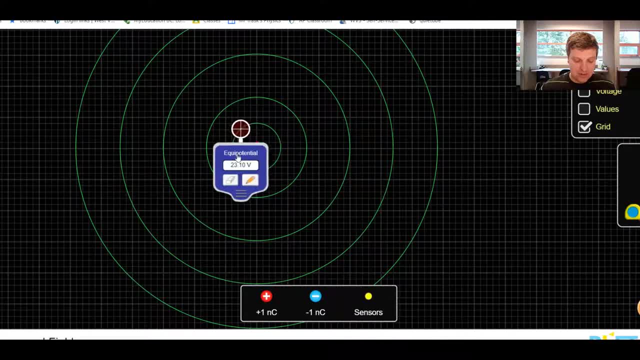 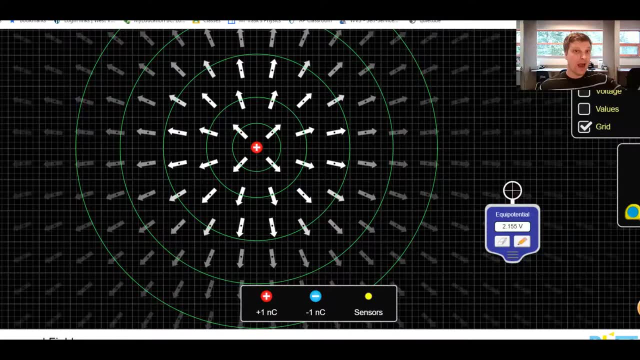 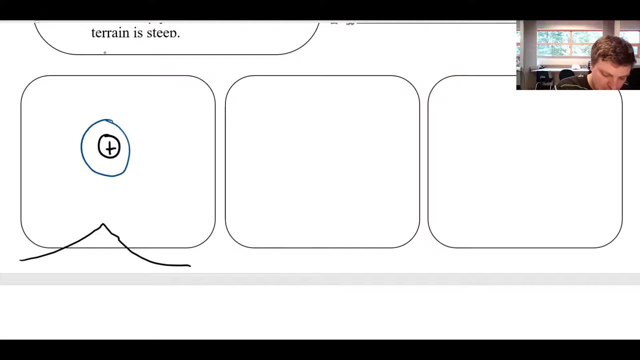 anywhere on this line, bring this back here. if I say anywhere on this line, I can see that I'm staying at the exact same voltage. it's like walking around the top of the mountain but not actually going up or down the mountain. So this picture here, this equipotential line, would be just these concentric if I could draw. 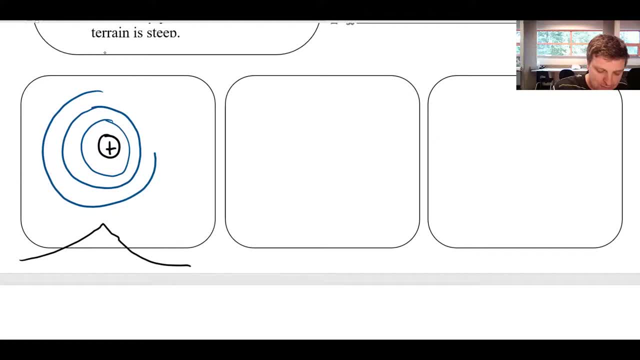 concentric circles, I would imagine, if you will, nice looking circles. so then what would it look like if I did the same thing with a negative charge? well, I guess a negative charge would be the opposite situation, where it'd be like a really steep valley or something like that. that would be. 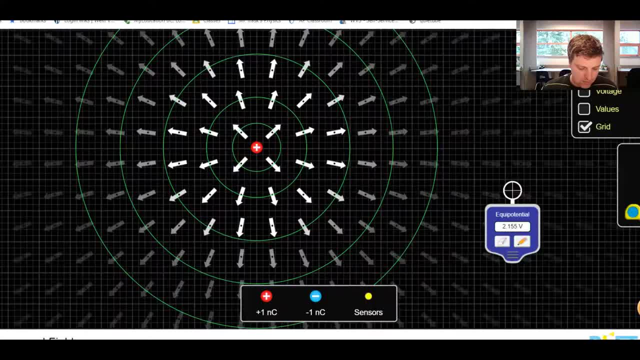 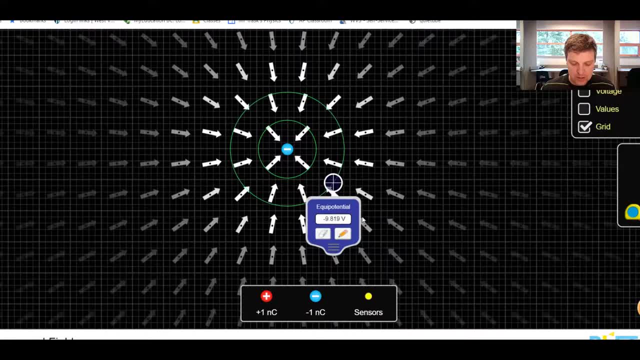 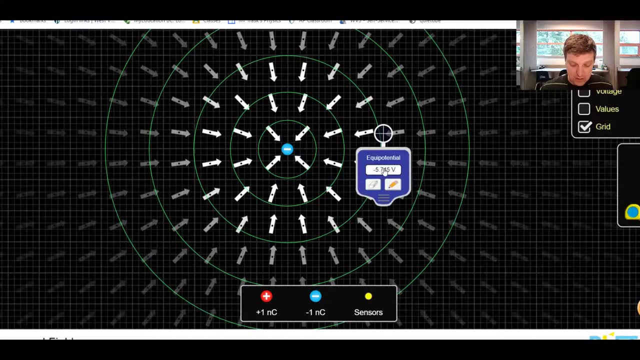 like a really low potential, and so if I jump over to my simulation here again, I move in my negative charge and I add some equipotential lines, we can see that. well, actually it looks exactly the same. these are low potential, these are negative potentials, like when I walk around in this. 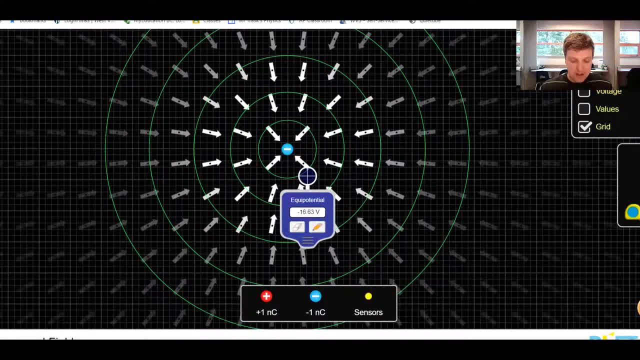 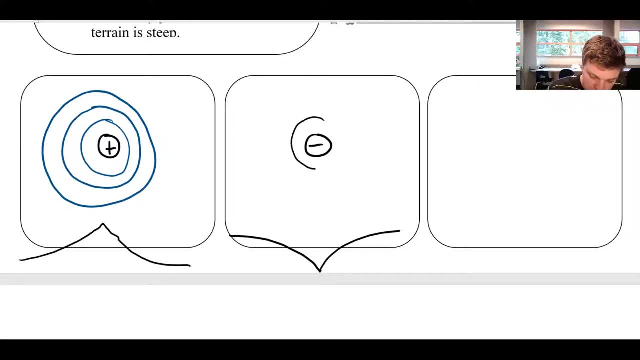 space I can see I'm staying at about negative 20 volts, but from the top view the kind of equipotential lines sort of look the same, and so I might just draw again somewhat concentric circles while you visualize perfectly concentric circles. so what happens if we combine these together? what happens if we have multiple charges in the same? 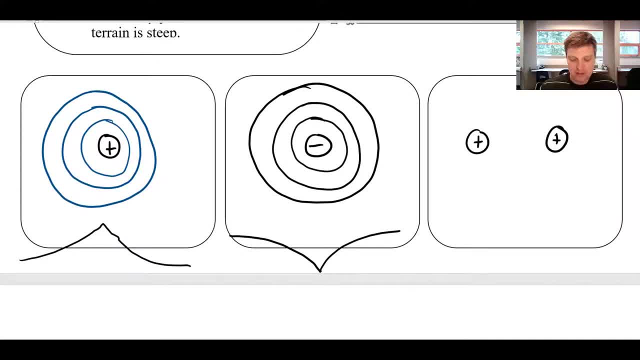 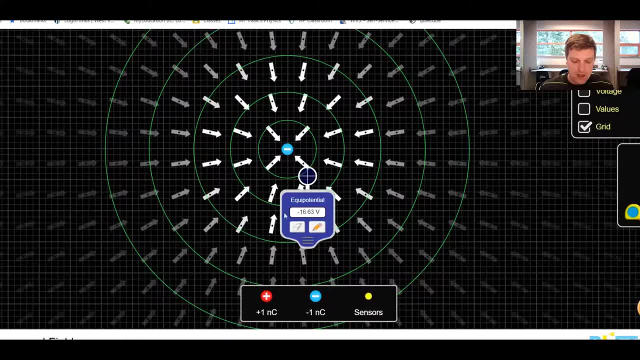 space. and I encourage you to kind of think about this and maybe even hit pause in the video and kind of sketch out what that picture might look like, or just sketch it out with pencil and then go back and see if you got it right, because when we have two of these positive charges, kind of near 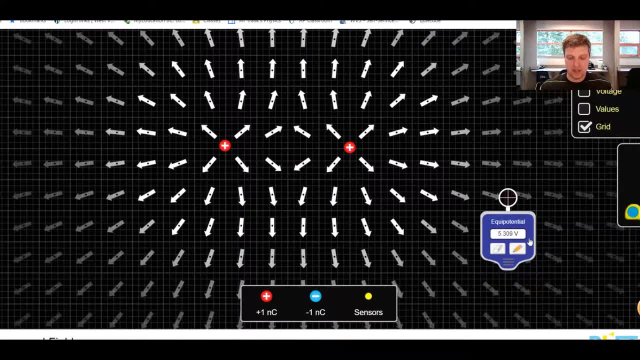 each other. they're both kind of like making these areas of high potential, these mountaintops. if I'm close to this one, that looks like a kind of like a perfect circle. again, I'm not sure if it is or not, but you can see that it's kind of like a perfect circle again I'm not sure if it is or not, but you. 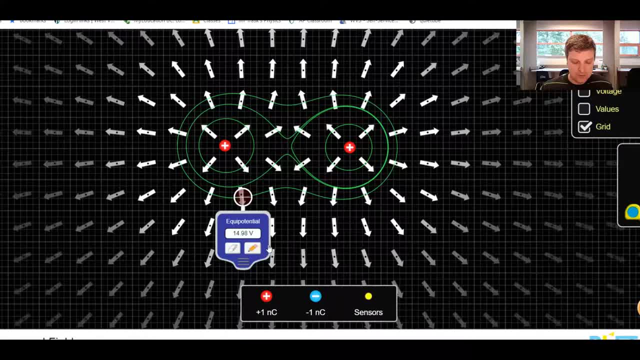 can see that if we go a little further away, eventually we get to this space where it goes around both of those, because if you have two really high mountain peaks, it makes sense that as you get further from that mountain, eventually there will be a line where you can walk around. 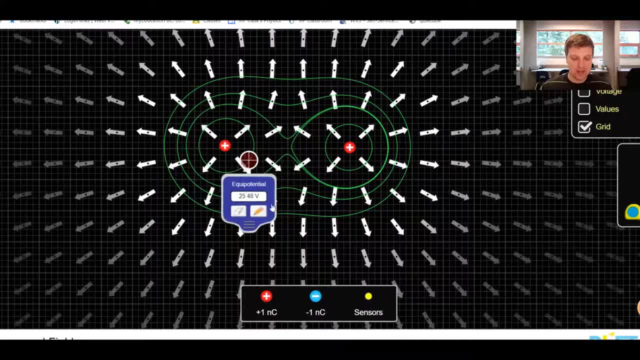 both of the mountains without having to climb up or down. when you're really close to this one mountaintop, you could only walk around the one mountain. you'd have to climb down in between and back up to get to the other peak. so this picture is going to kind of. 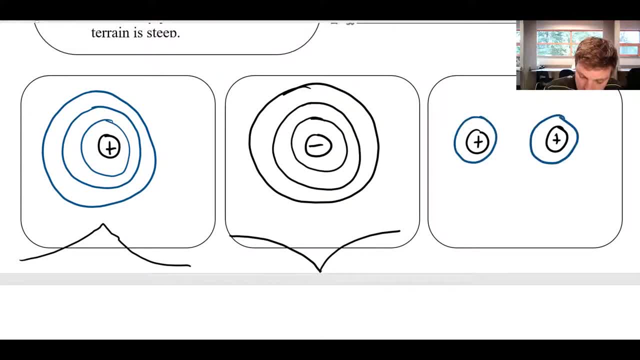 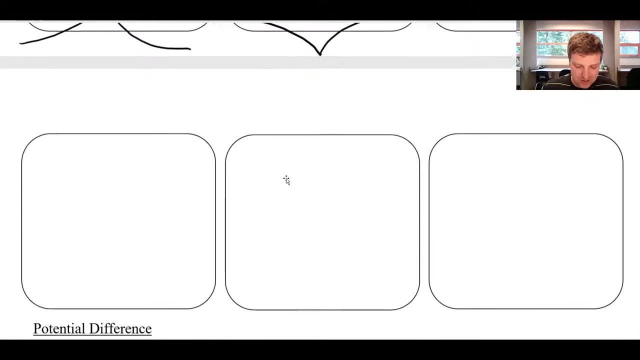 look like this. so here's a real test of my artistic ability. it's going to kind of look like this, and if those were exactly equal charges, then that would be a more exactly equal symmetrical looking picture. but um, as we know about my art skills, they're. 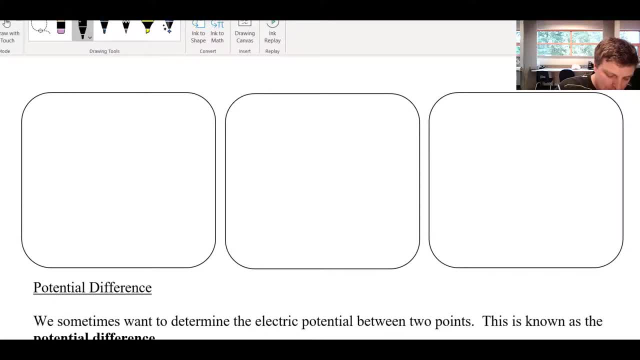 they're still in progress. so, um, what happens there if I, what happens if this charge here I'm gonna make like a plus three charge and I put this near like a plus one? what would happen if I, if I kind of supersize my charges and again, um, go ahead and, just you know, think about it for a 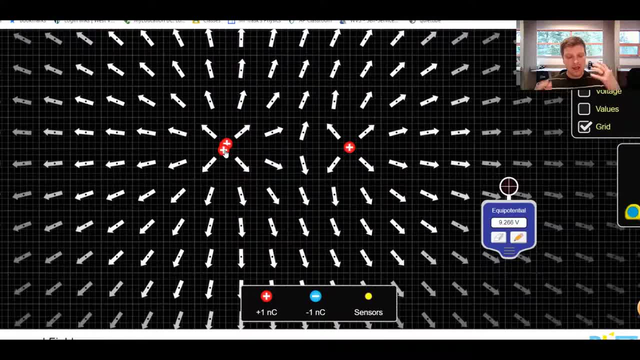 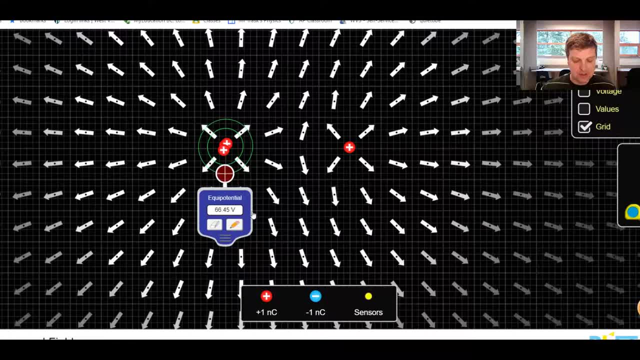 second, I'm going to add in these more charges here, so I've got three charges there. kind of visualize what's going on there, think about what, um, what this might look like when I'm close to this mountain. this is very much still kind of concentric circles, and I'm close to that one. 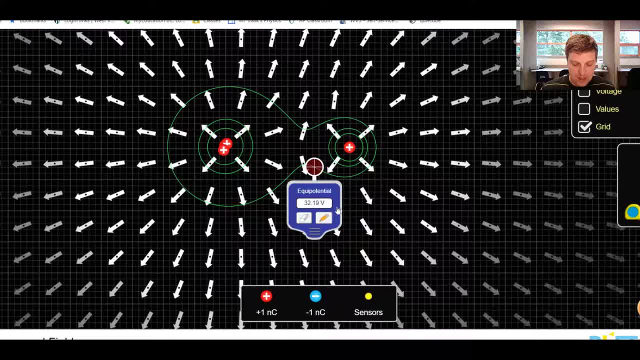 it very much looks like circles, but as I get further away we can see that we get to a point where actually this one here, I'd have to be much further from this mountain in order to be at the same potential as when I go around this one, I can be closer to this mountain and stay at the same. 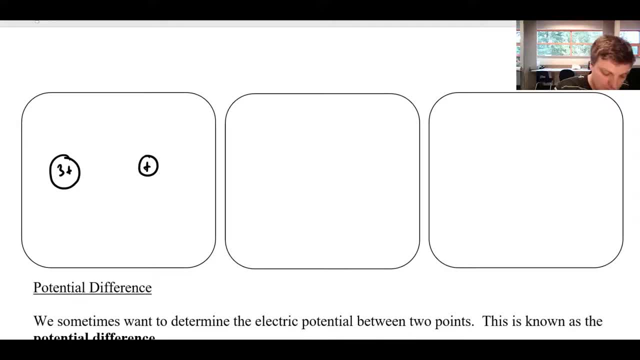 potential, because it's a smaller mountain top, if you will, and so this potential line would kind of go, maybe just around here and this one goes kind of just around there, but then this potential line that goes around this one is going to go all the way around. this one kind of like this idea here. 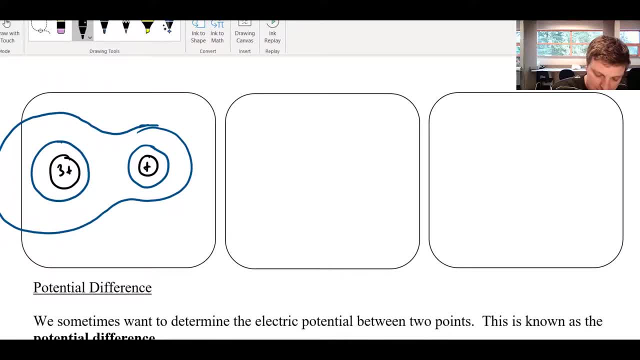 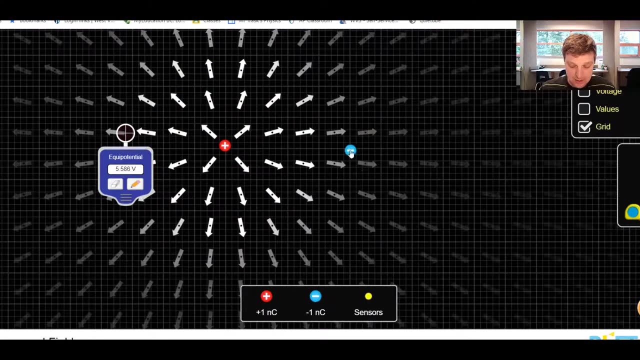 okay, we might just do one more, just to just to solidify things. so what happens then? if I have a positive and a negative, um, and I've got a plus and a minus, and so, uh, let's get rid of these extra positive charges here, and let's get rid of that positive charge, and let's add in here a negative charge. 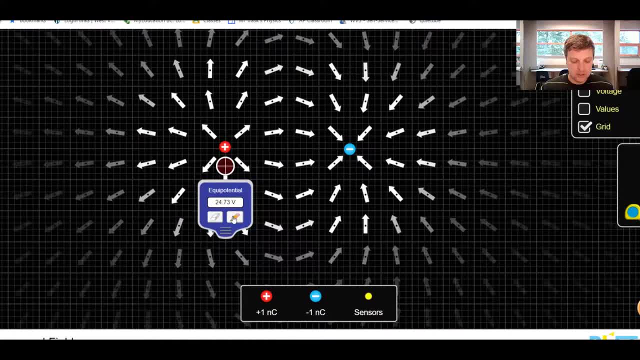 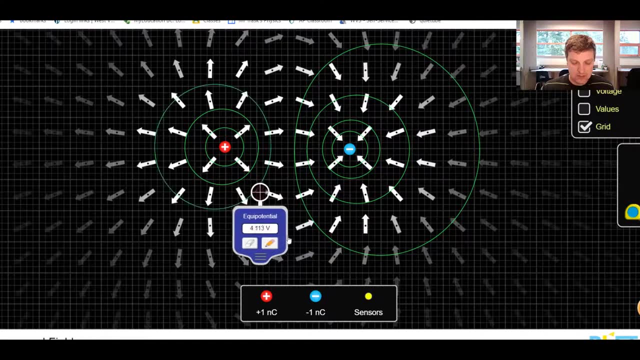 so what's this going to look like? well, um, close to this is going to look like, um, the peak of the mountain and close to this is going to be kind of the bottom of the valley. but as I get further and further away, these circles are not going to stay concentric and they're not actually. 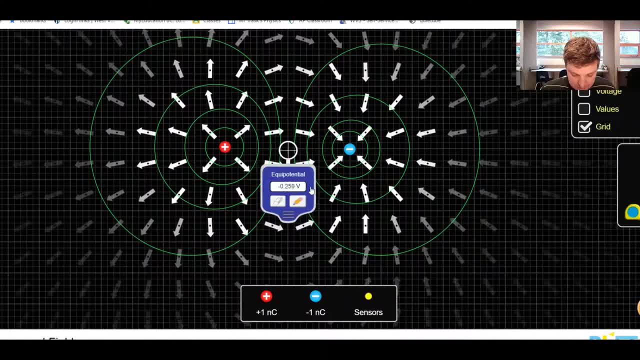 circles at all and if I can get it right. I probably can't get it perfectly right, but I'll try and get as close as I can. if I got it right in the middle, we might notice that there would be a line straight up and down. now, why is that? well, think about it. you can't get from the top. 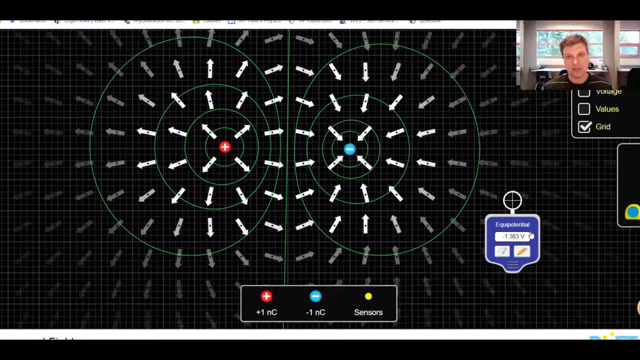 of the mountain. you can't get anywhere near the valley without crossing these lines. right, this point in the middle, here directly in the middle, would be at zero voltage because the mountain top is creating positive voltage or positive potential, the valley bottom is creating negative and those things add up, they would add up to zero and they would cancel each other out. 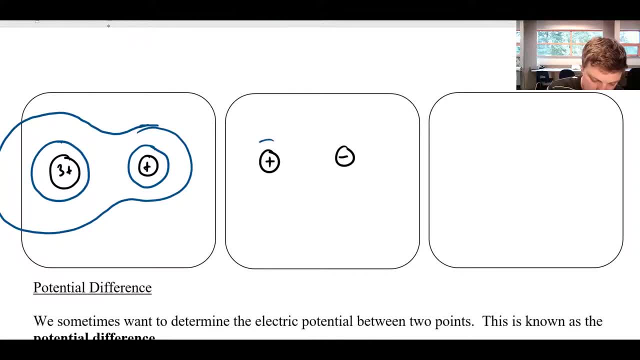 so this picture here would look kind of like this and this, but then maybe like a bit distorted that way and a bit distorted that way, and maybe I'd have a line right in kind of the middle together. so we got one space for one more. let's just do one more, why not right? uh, let's make. 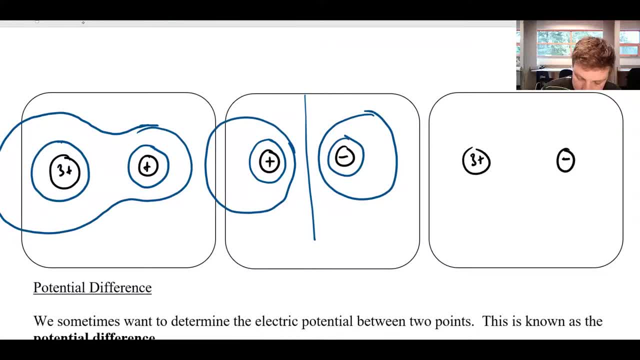 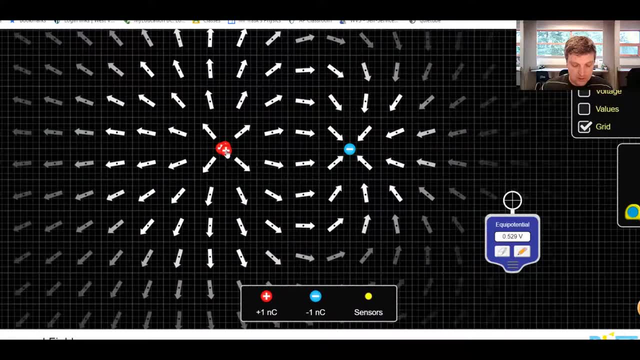 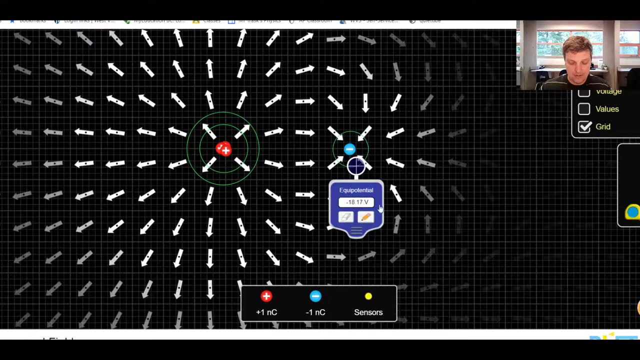 it a little bit more specific here. so I've got one here three plus and this one here one minus and what's that gonna look like? so I'm gonna add in my extra positive charges to this space here. so I've got a pile of positives. so I can see that here I've got my kind of mountain top and there 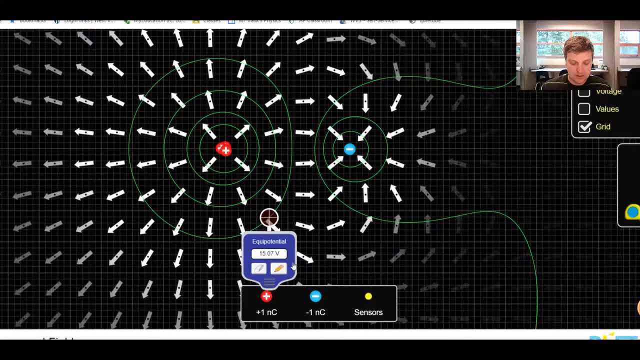 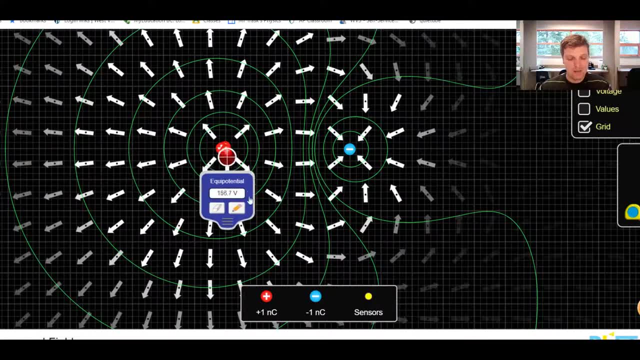 I've got the valley bottom, but as I get further away something kind of funky is going to happen here. let's see if I can decipher what's going on so you can see that essentially what happens is this: positive charge is so strong that the point where we'd be at zero voltage first of all. that's much closer to the negative charge, but it even 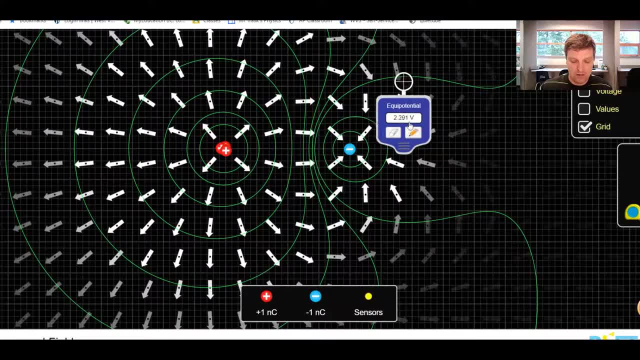 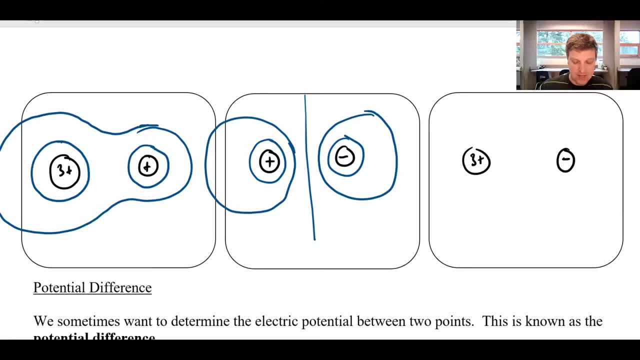 extends off into space, so zero voltage would happen way over here and around here. it's like you can see that this positive charge is almost like it's taking over the- uh, the space in that sense. so I've kind of got, um, kind of got concentric circles there and there. but then this: 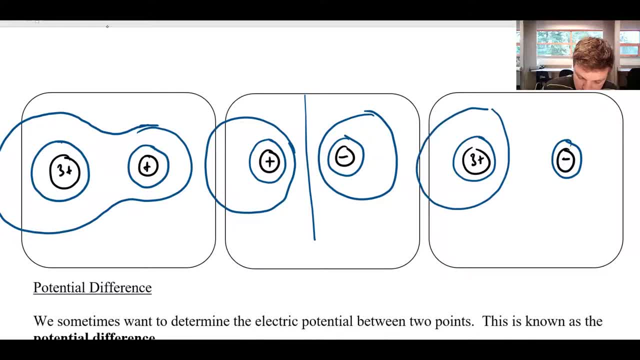 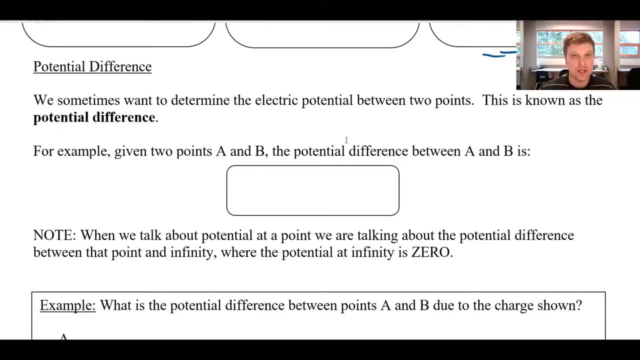 goes like this and then it kind of goes like this and takes over everything and kind of running out of space, so something like that. okay, so when we talk about potentials, just like we had with uh energy, we can have changes in energy, we can have differences in energy, we can have differences in. 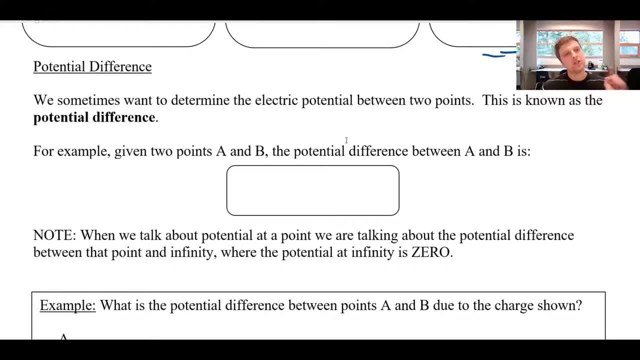 potential. it's often useful for us to know not just what's the potential at one point, but what is the difference in potential between two points. this, this point, is this high in potential. this point is this high. I know I'm going to have to do work to get that proton up to there. or I know, for example, that an electron would want to just 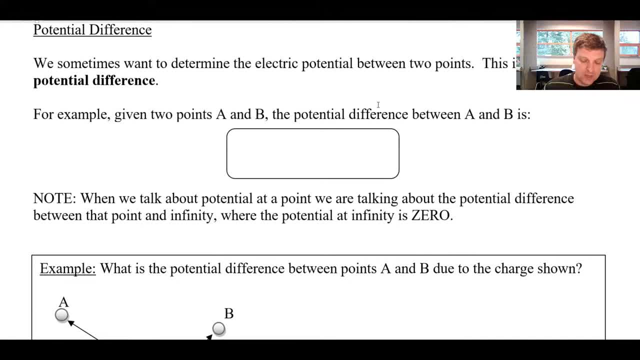 go there without any work at all, and so the difference between two points, the change in potential between two points, would just be, in this case, vb minus va. so if I have two points, a and b, the potential difference is vb minus va. it's like the fi, the point you end up at, minus the. 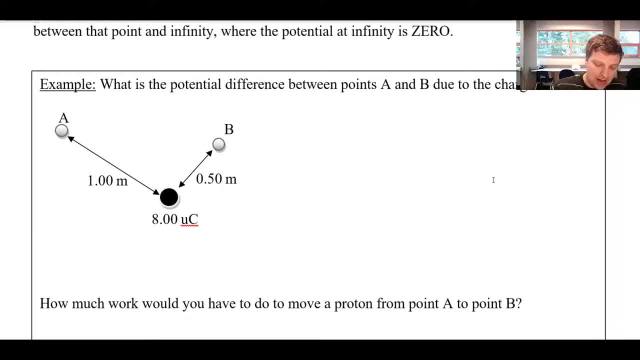 point you started from. so imagine that I'm wondering what is the potential difference between points a and b? okay, so I can find. for example, delta v is just going to be vb minus va. so, knowing my formula for potential, I could just say this is k times q over rb minus k times q over r a, and notice that the charge here is the same charge. 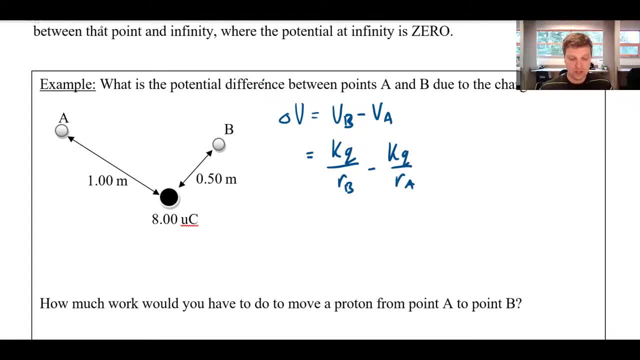 we're not changing our charge. this one eight microcoulomb charge is going to be the same charge. we're not saying that this is the negative charge. that's going to be the negative charge, and so what I'm going to do is I'm just going to subtract that and you can see here that we've got. 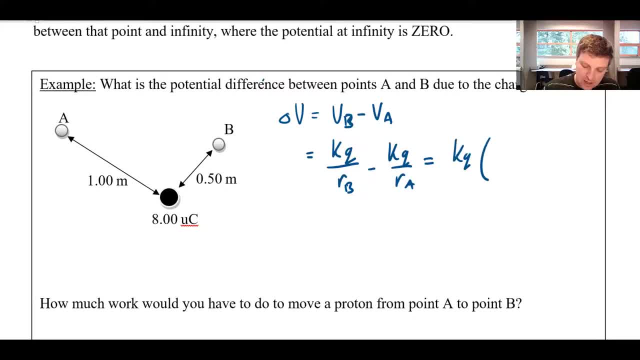 a common factor of kq, so I could write this as kq times 1 minus rb1 over rb minus 1 over r a, and so, subbing in my values, I get 9 times 10 to the 9. multiply that by the charge 8 times. 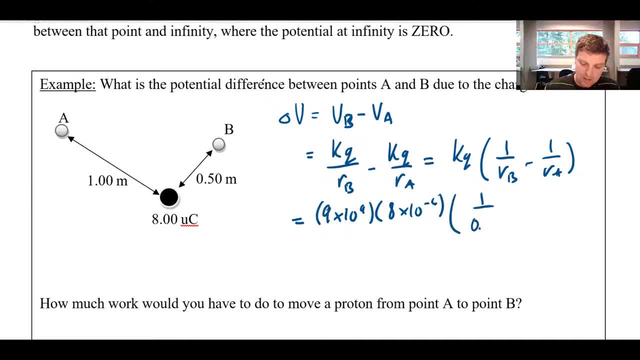 10 to the negative 6, and then don't forget to do the inverse: 0.5 minus 1 over 1.0, and so the potential difference between these two points ends up being 72,000 volts. is the potential difference between these? Now, when we talk about a potential difference, we haven't done any work. 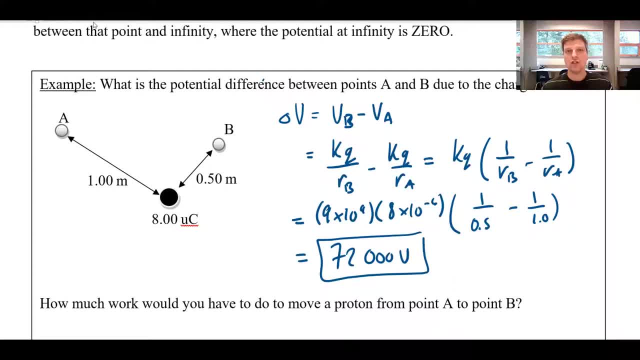 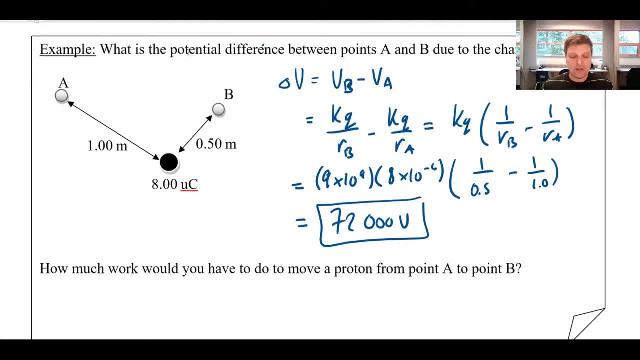 yet We haven't moved anything from A to B, So there's no energy involved. We're just saying: basically, point B is 72,000 volts higher than point A. That's all the information we have. But where that's useful is if we now come along and say: okay, how much work would you have to? 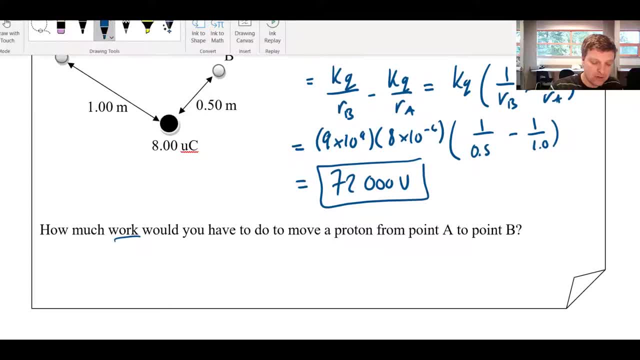 do to move a proton from A to B? If we actually want to move something through this space, how much energy is this going to take? Well, work in this case being my change in potential energy potential, energy potential being defined as potential energy per unit charge. 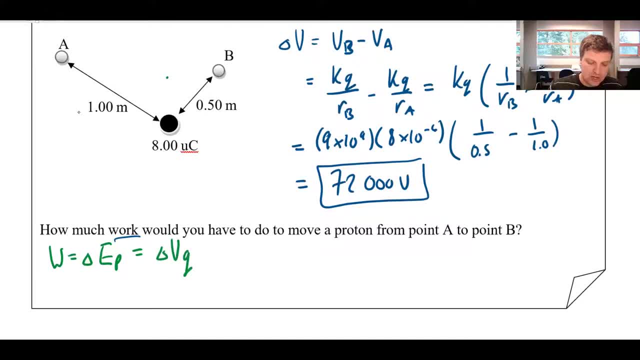 that means my change in potential energy will just be my change in voltage times the charge. So my 72,000 volts multiplied by my positive charge of positive 1.6 times 10 to the negative 19 coulombs is going to come out to be 1.15.. 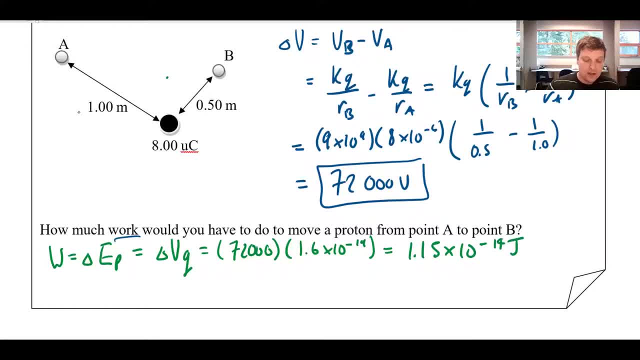 Times 10 to the negative 14 joules. Now I want to point out- maybe not a great example, but this is plus 72,000 and this is plus 1.6 times 10 to the negative 19 coulombs, which means that 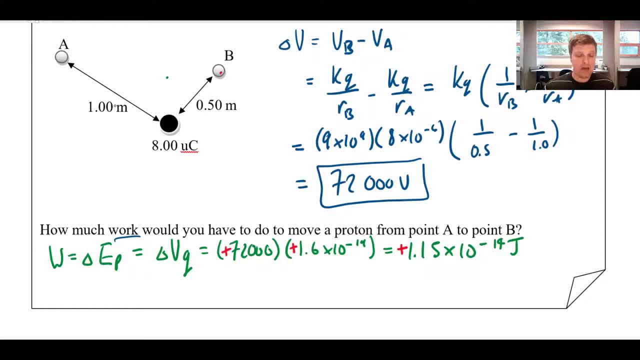 my work came out as positive as well, And that's because I would have to do work on this proton to move it over here. It doesn't want to go there. I'd have to add energy to the system to move it along. So if, for example, I had done the same calculation with an electron, I would have used 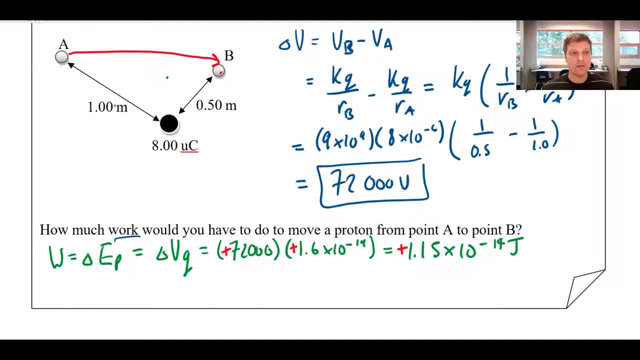 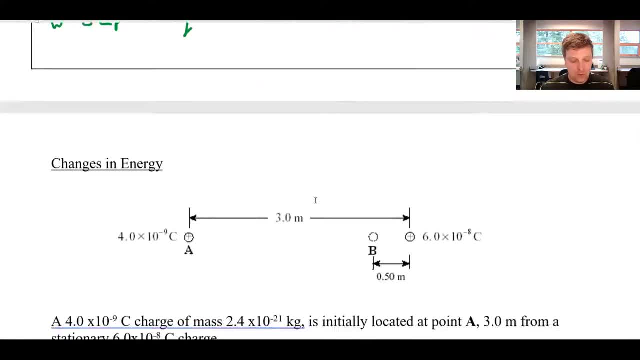 a negative charge and then the work would have come out as a negative value, because the electron is very happy to move there. for me It's happy to release that energy as it goes. Okay, So we'll look at one last example here with changes in energy and bring it all together. So imagine I've 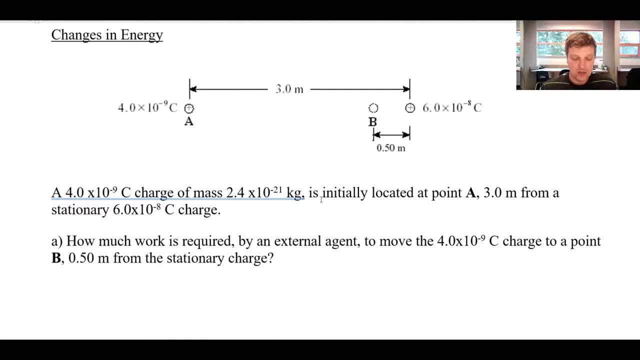 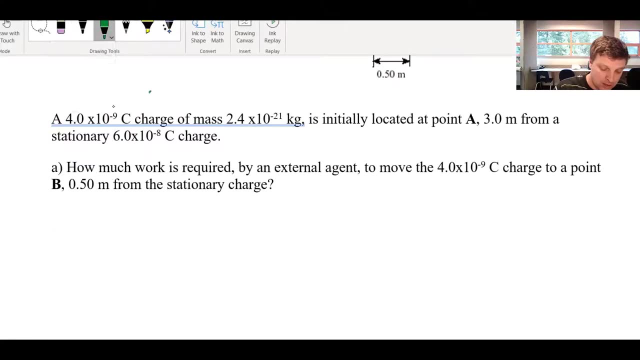 got a four nanocoulomb charge sitting here at point A and I'm going to compress it into point B. So I'm going to do a bunch of work on this system to compress it over to point B. How much energy is going to be done on that charge to move to that point? Well, we know that our change in 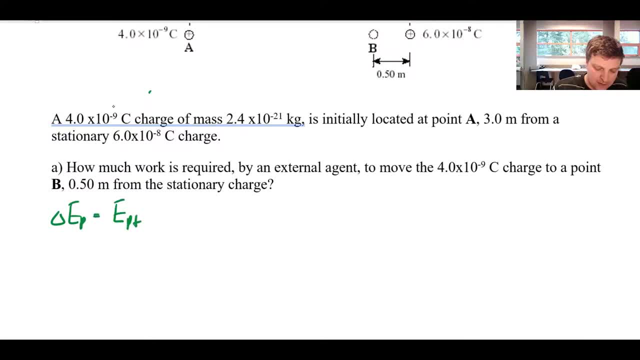 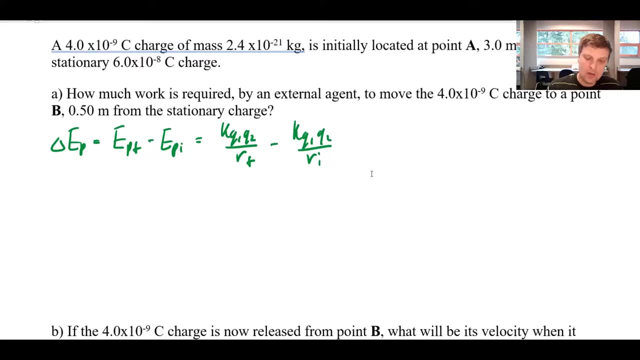 potential energy is just going to be E p- final minus E p- initial. Now this is going to equal k q1- q2 over our final, minus k q1- q2 over our initial. But that's a bit clunky and we can see here that we can collect some like terms and write this as k times q1 times q2 multiplied by. 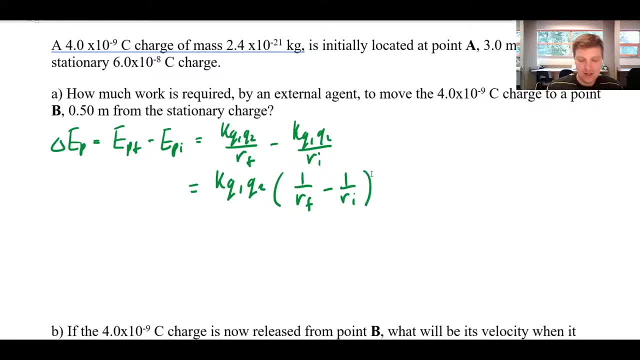 1 over our final, minus 1 over our initial Way. better, So much better, as you can see, And so now I can substitute in my values. But just think about this before you start plugging numbers in: I'm expecting that if I take a positive charge and move it closer to a second positive charge, 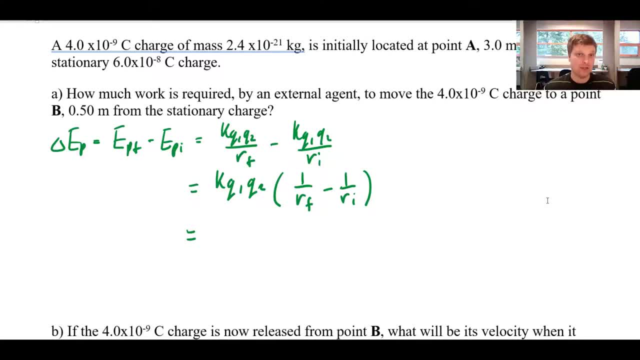 I'm expecting my change in potential energy should be positive. If I came up with a negative answer, maybe I've mixed up some numbers somewhere, So just be aware of that. So 9 times 10 to the 9. So the first charge is 4 nano coulombs And the second charge is 6 times 10 to the negative 8. 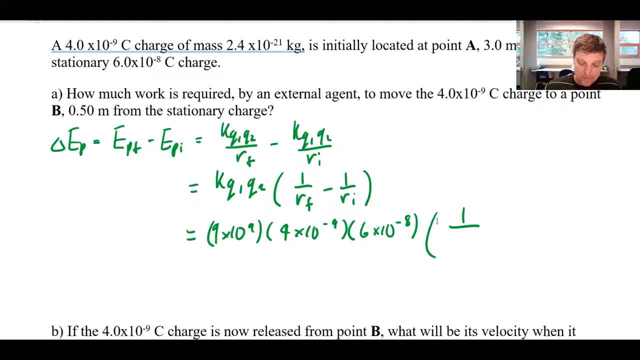 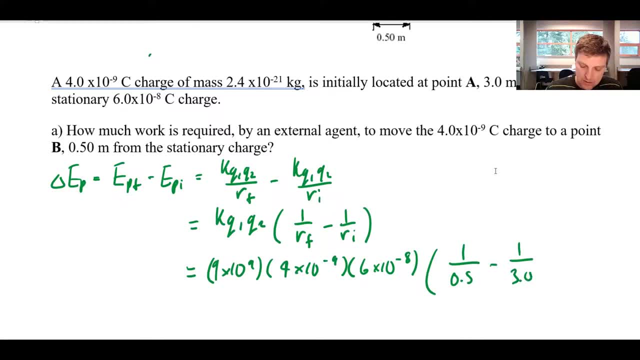 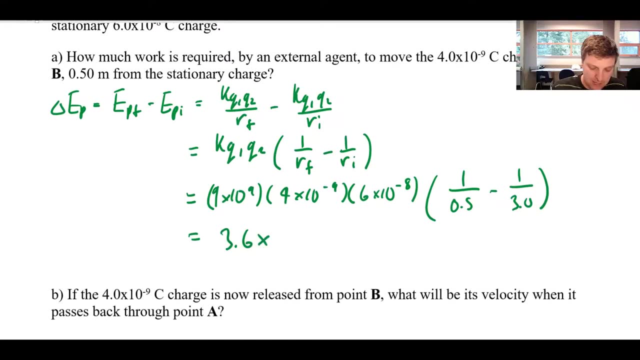 coulombs And I multiply that by 1 over, Remember my final is 0.5.. So 1 over 0.5 minus 1 over 3.0.. And my total change in potential energy or work would be 3.6 times 10 to the negative 6 joules. 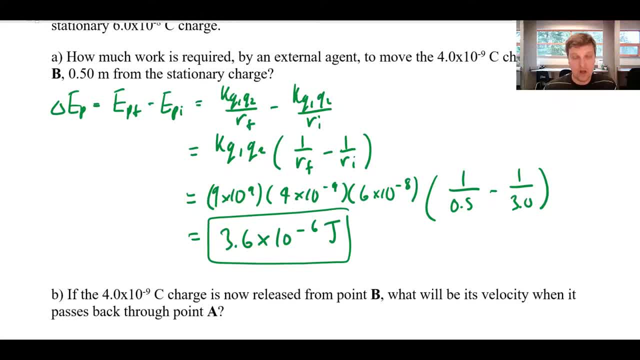 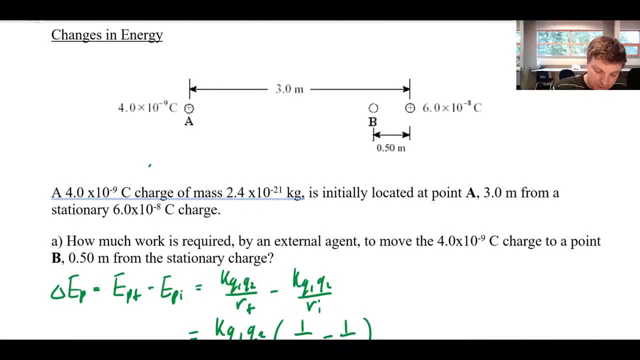 And I got a positive number there, So that makes sense. I'm a little confident in that solution. So then now imagine what we're going to do is here. We did all this work, So we did a bunch of work to kind of compress this over. 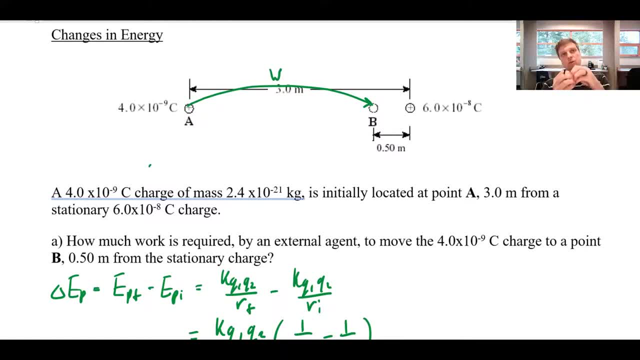 here, We put it in that space, And now what we're going to do is we're going to release that charge. So we now release that charge from this point And then, of course, once we release that charge, it's going to be very happy to go flying back in the opposite direction, because it has all that. 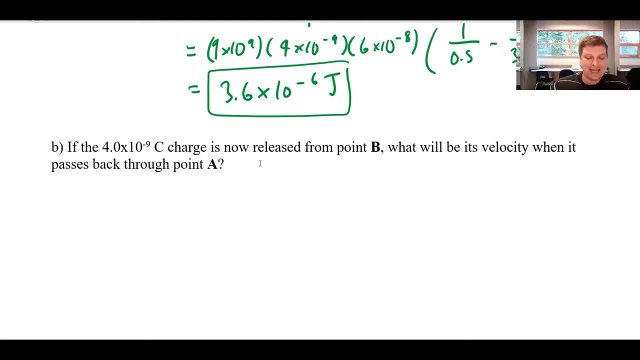 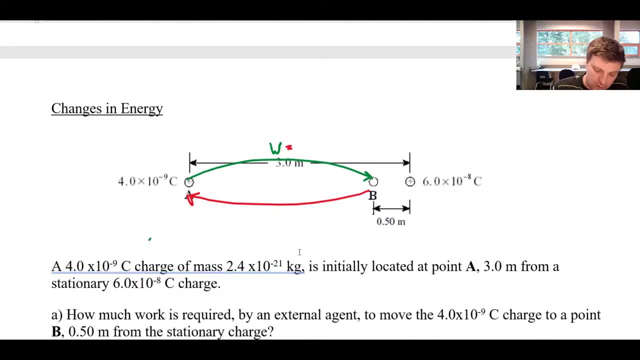 stored energy. So it says: what will the velocity be when it gets back To point A? Well, the energy that it gained when you did work going forward. So this would be like a change in potential energy. that was a positive. When it flies backwards, my change in potential. 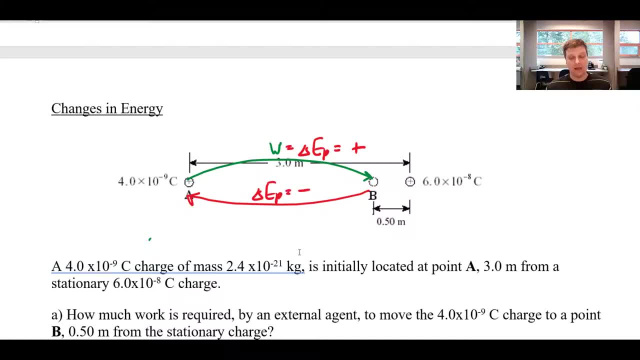 energy will be the exact same amount, but negative. So the exact same. what was it? 3.6 negative 3.6 times 10 to the negative 6 joules is what's going to be released as it flies back to. 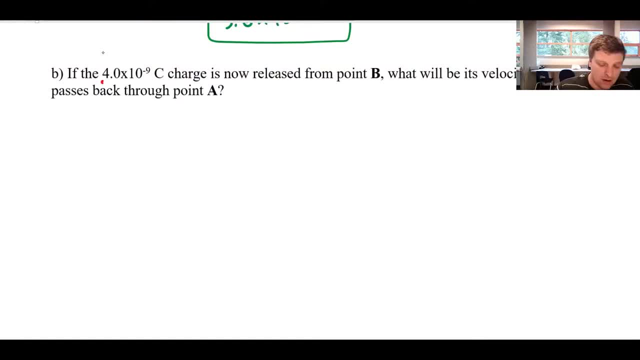 that point, And you'll remember that our law of conservation of energy says that a negative change in kinetic energy is going to be equal to a negative change in potential energy, And so basically, all that kinetic energy that we just lost is going to turn into kinetic energy. So negative times negative. 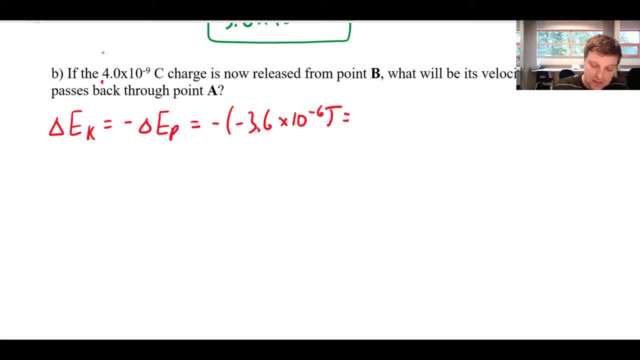 3.6 times 10 to the negative 6 joules basically means I'm going to gain 3.6 times 10 to the negative 6 joules of kinetic energy. It's a little bit convoluted, but if you keep track of your. 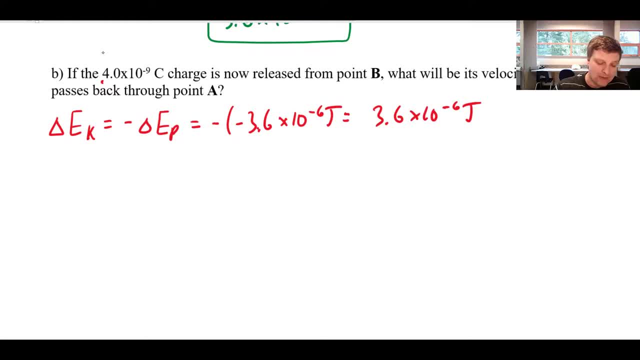 positive, negative signs, you'll be okay. So if I'm gaining that much kinetic energy, then I know that my change in kinetic energy would just be ek final minus ek initial, where that initial kinetic energy is also zero, And so really it's just equal to my final kinetic energy. So the final kinetic energy.